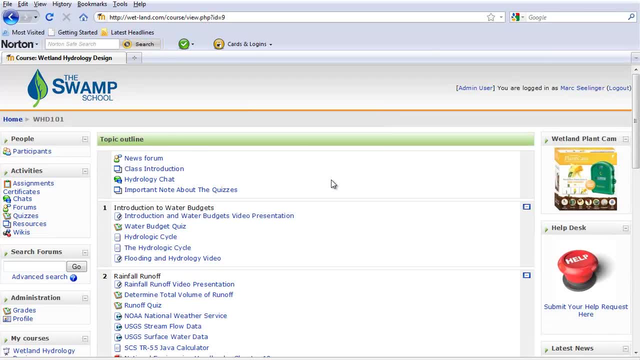 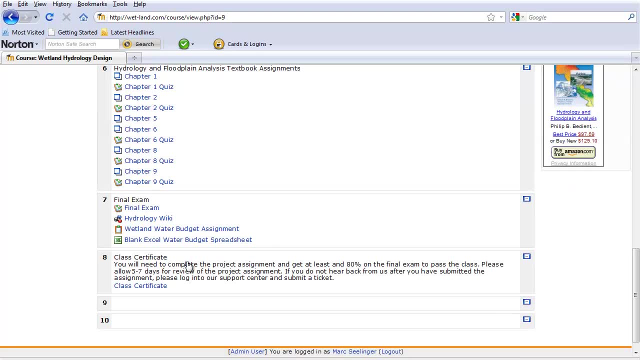 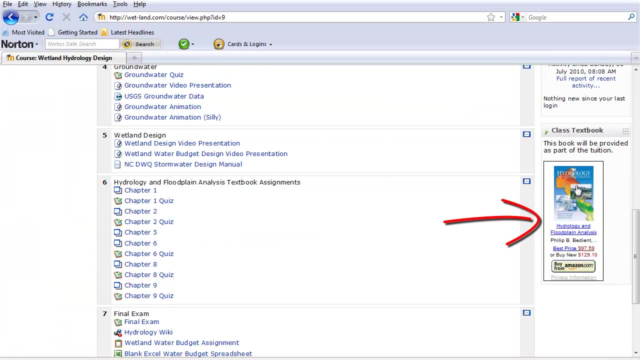 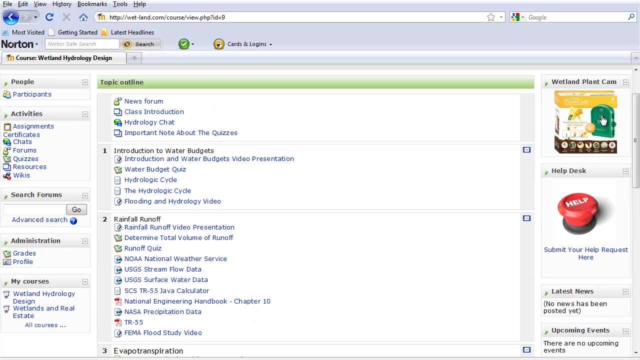 the topics And, as you can see, we have things: introduction of water, budgets, rainfall, runoff calculations, evapotranspiration, groundwater design, hydrology, then the final exam and some certificates and other things like that. There's some resource information on the side. here. There's an example of the textbook. This does come with the class, but we do give you at least a sneak peek at that. A couple of promo stuff here on the side: Your grades courses that you're signed up for. 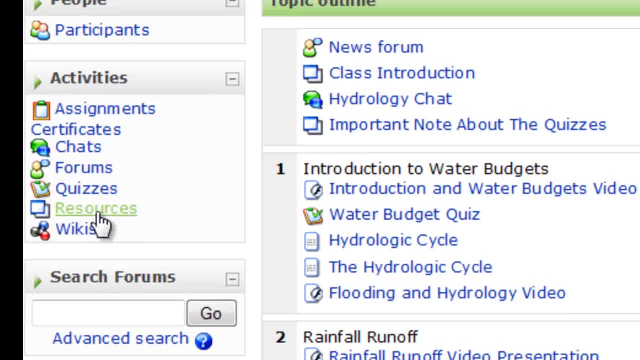 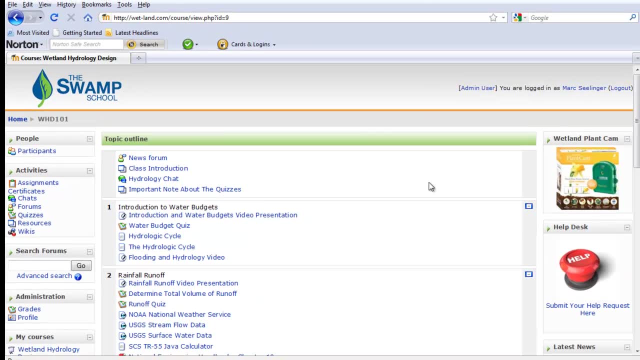 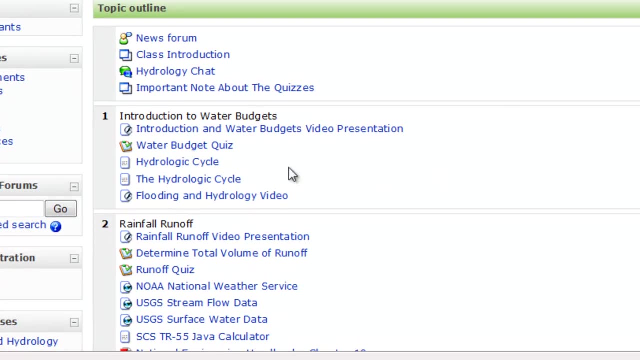 all this stuff is in here. We have chats, forums, wikis, all kinds of other resources here so that you can take a look at it. If you want to take a look at who else has signed up in the class at the time, you're also in there as well. Now, to give you a quick rundown of what you can expect, you'll see that most of these topics kind of follow a standard procedure here. We have, for example, introduction of water budgets. We have a video presentation- We're going to give you a quick quiz on that- Some resource material on the hydrologic cycle, Maybe even an additional. 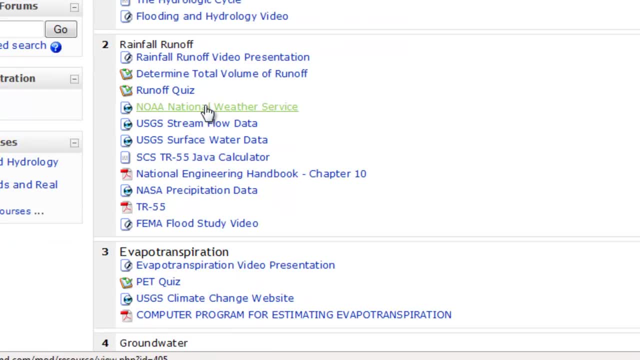 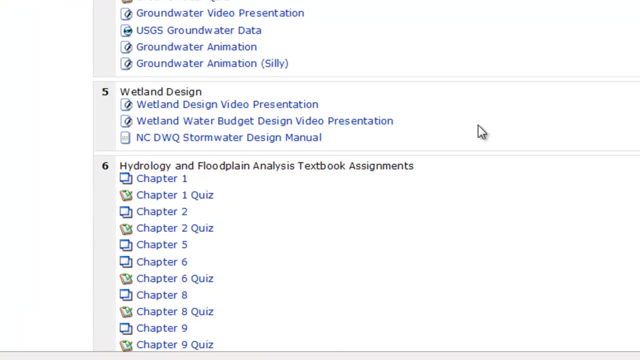 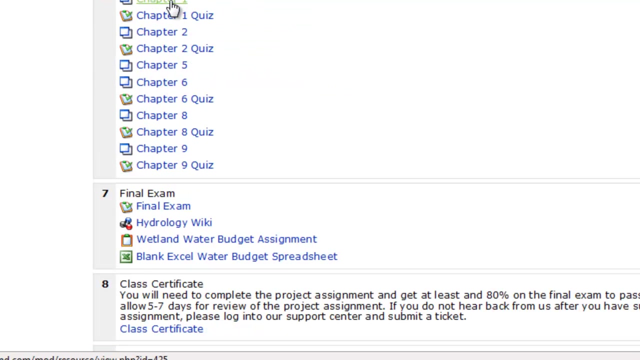 video presentation through here And, as you can see, some different sources here. The little F here is the flash format If we link you up to another site: stream flow data, surface water data, some calculators, We've got PDFs in here, Lots of different stuff again going through this. Now we also get to the textbook assignments, because we do have textbook, And each one of these what we're going to do is give you, for example, pick chapter five here We might have a section on here where we're going to give you a little bit of information about the textbook. 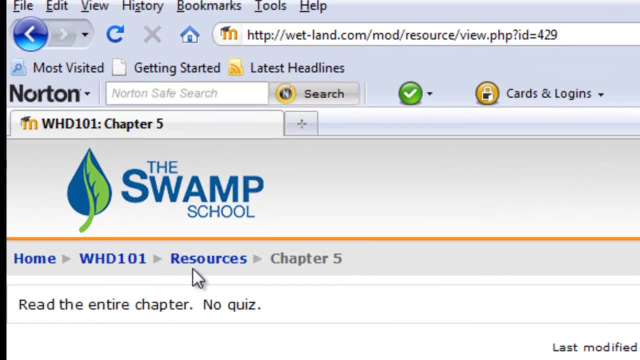 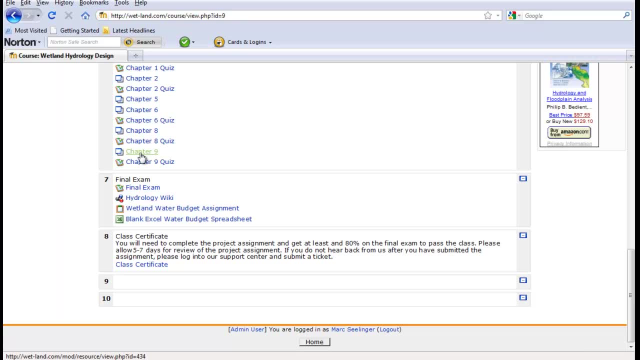 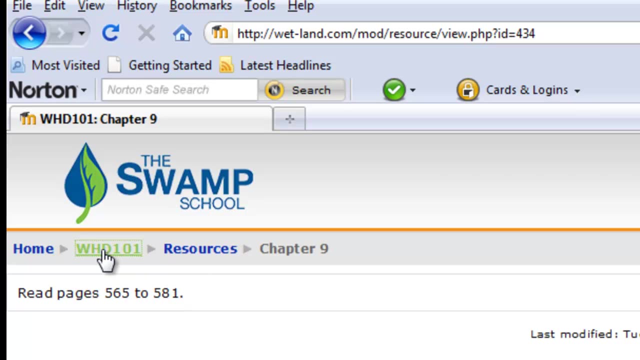 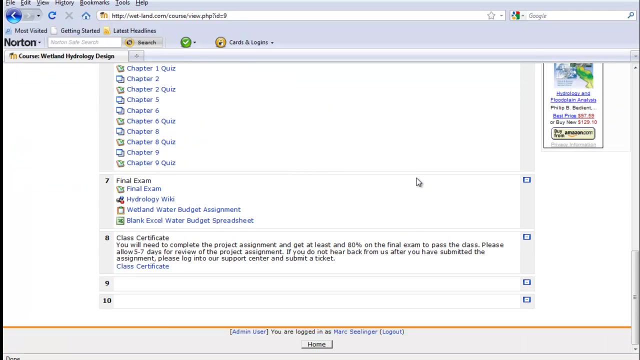 Which you can basically read the entire chapter, but there's no quiz. So we're going to give you an idea of what's there. Other sections: we may just have you read a section of the chapter, And it's just going to be page 565 to 581.. So we don't need to cover the whole thing, And then the quiz is just going to be some specific questions related to that. So you'll have that as well. So you're in good shape there To give you a quick sample of what one of the videos looks at. let's just pick one. How about you? 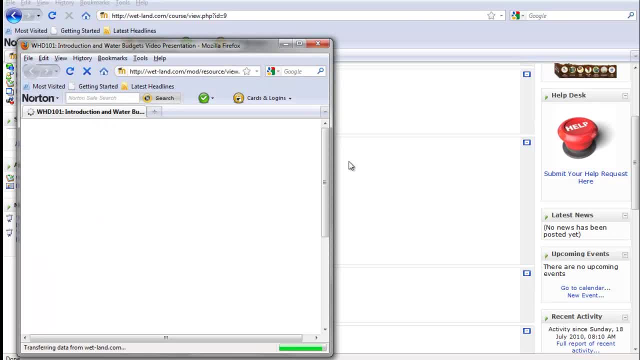 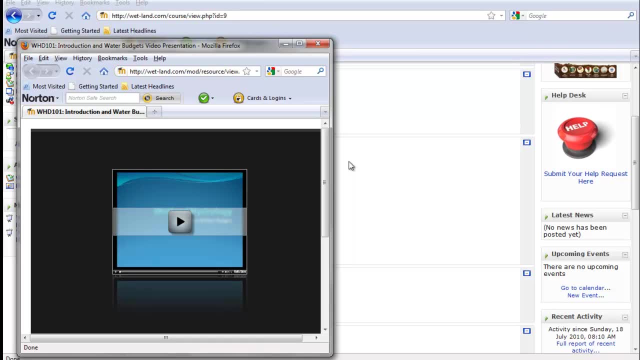 Not just the introduction one here. So let's just run this real quick. All you have to do is click it. It is Flash, So it's going to require that you have your Flash player, which is a free plug-in, But that does need to be installed into your browser, And then, once that comes up, you're just going to click this and it's going to play. So I'm just going to click this real quickly and give you one or two slides. 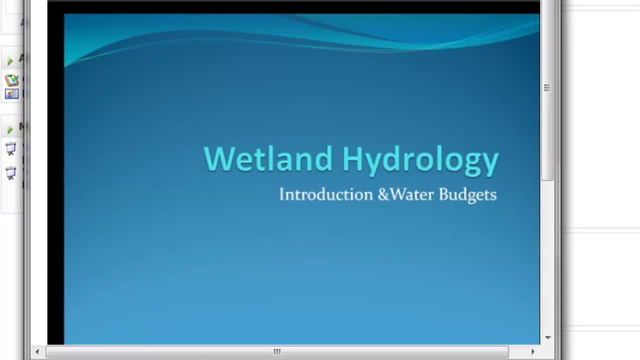 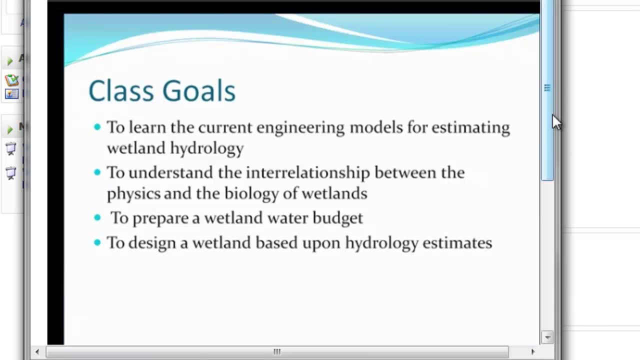 Hello and welcome to the wetland hydrology section. Today we're going to be discussing water budgets and some background information on wetlands and their hydrology. Our goals for this class are to learn the current engineering models that are used to estimate wetland hydrology. We need to understand the interrelationship between the physics and the biology of wetlands. We need to prepare a wetland water budget And, finally, we want to be able to design a wetland based upon these hydrology estimates. 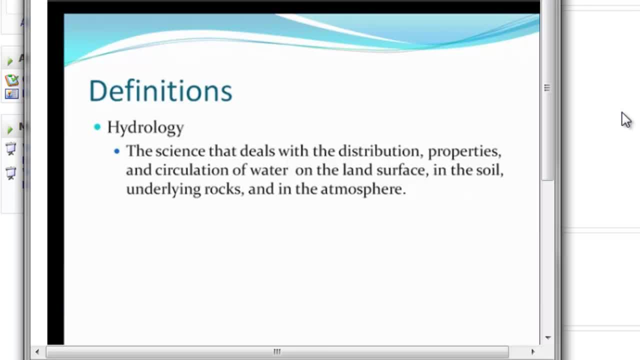 So what is hydrology? Well, it is simply the science that deals with the distribution, properties and circulation of water. This is on land, This is in the soil, within the rocks, in the atmosphere, in the snow and anywhere else you can find water. So what is hydrology? Well, it is simply the science that deals with the distribution, properties and circulation of water. This is on land, This is in the soil, within the rocks, in the atmosphere, in the snow and anywhere else you can find water. 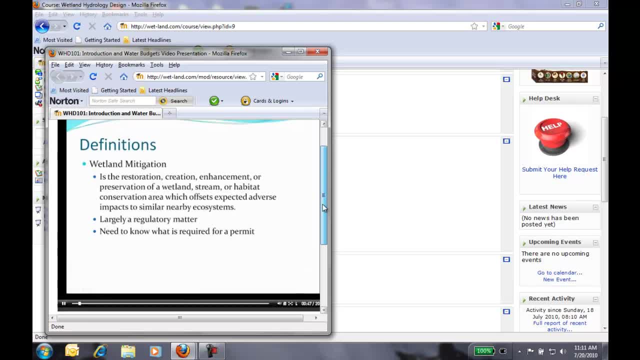 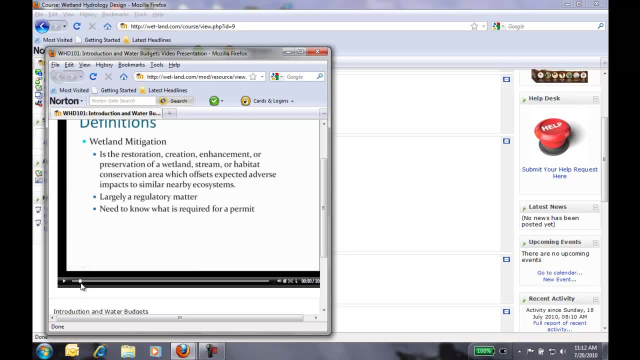 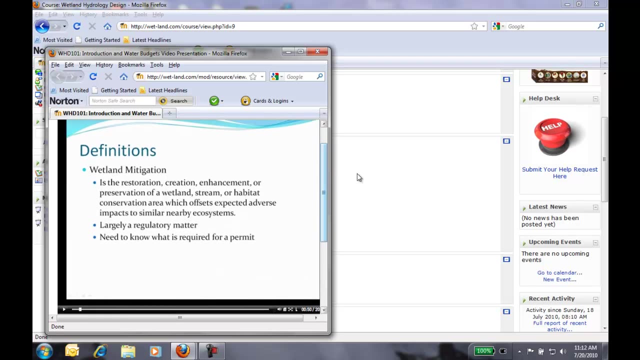 now what you can do here. as you can see, i stopped the video. you can. you can bookmark it. it does give you the ability to go back. so if you know the phone rings, you know you need to go back. you don't have to listen to the whole thing. it does run automatically and then you 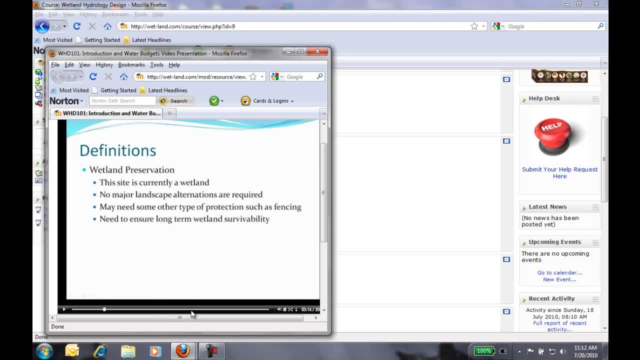 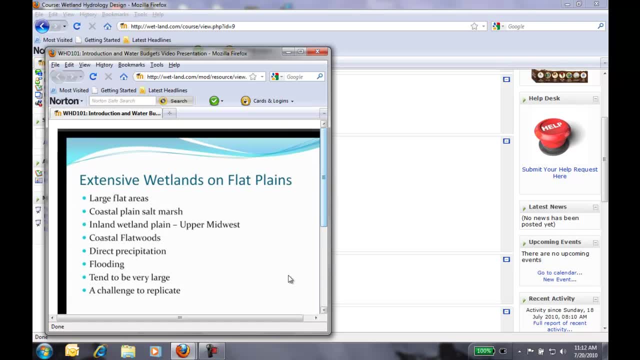 can just stop and pick up and you can slide. you know, as you can see, we can just skip around here and cover different areas and the video will follow through that. so you're you'll see the timeline here. this one's about 20 minutes long, so it'll give you kind of an idea also how, what 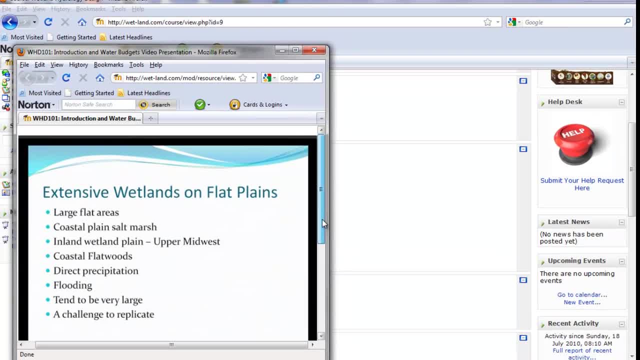 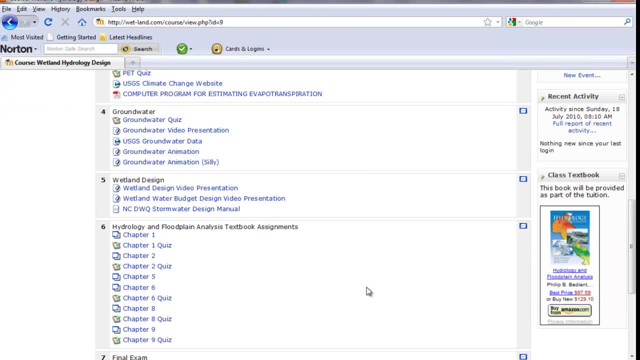 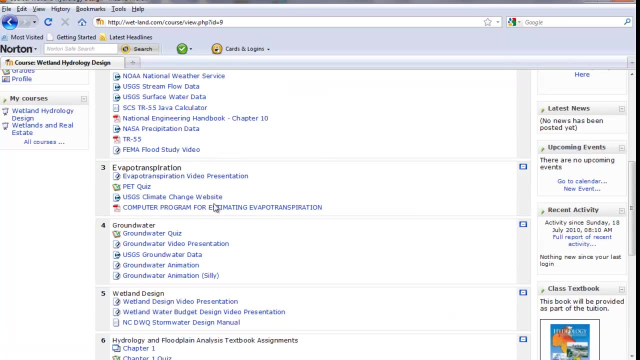 what you're in for it's when you get started, so that gives you a quick heads up on those, and each one of those is is is in here as a flash video. the other resources that you might find here- for example with the, the quizzes, we can run through a quick quiz here. let's try the. 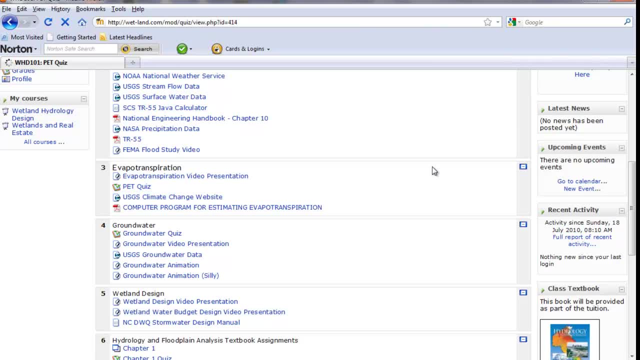 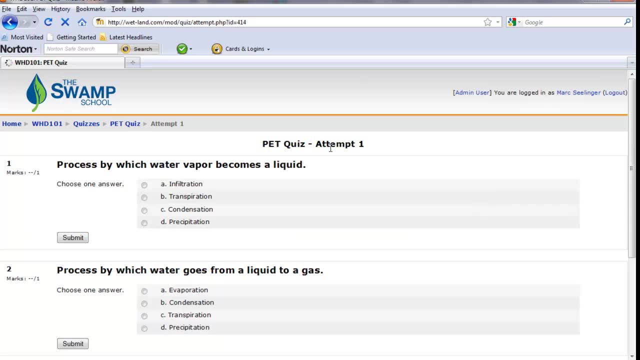 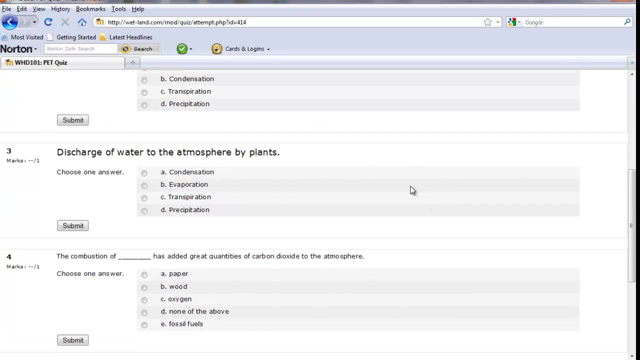 potential evaporation, transpiration, evapotranspiration quiz, and it gives us an attempt to quiz. now we click this button and it's going to ask us some questions, and most- most of these are a either multiple choice. sometimes they're fill in the blank. it's a variety of different types of 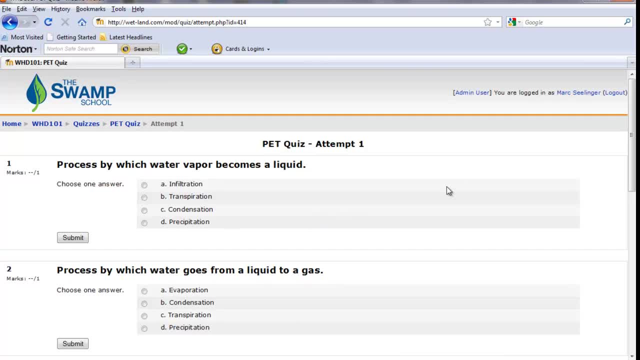 questions. there is a question bank that these things are feeding from, so if you do this, you're given multiple tries at the quiz, so you're not going to get the exact same quiz every time you run through this. you'll get several different questions, so you'll get some feel for that and 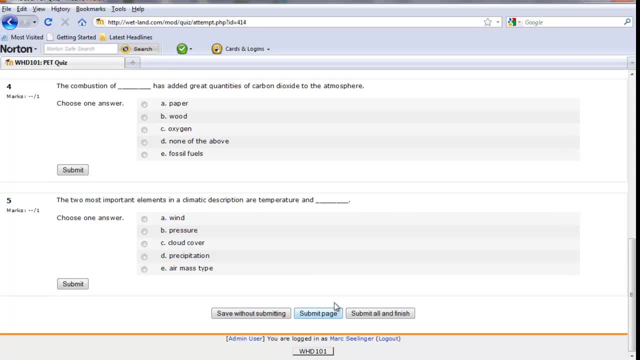 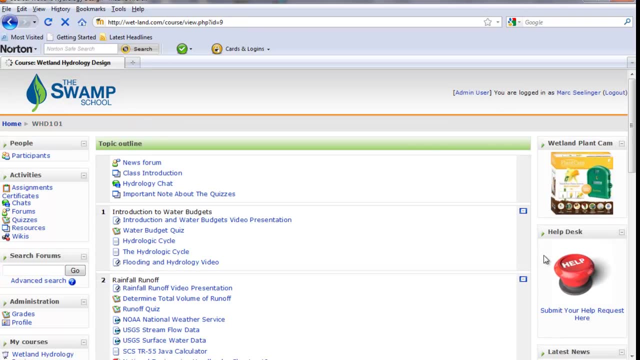 then you can submit, you can save without submitting, you can come back and change your answers whatever. whatever works for you. the goal of the quizzes is not to intimidate you with a whole bunch of hard questions, but basically to reinforce the learning and kind of get you to. 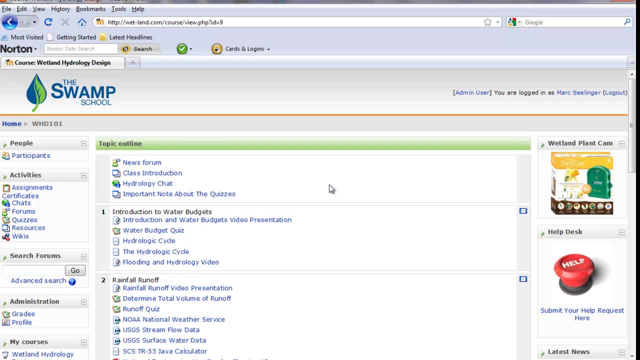 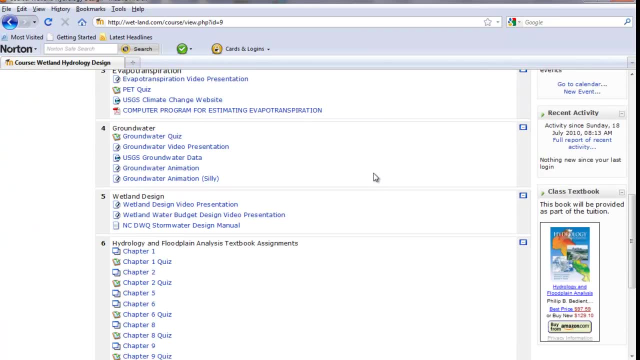 highlight on some of the questions. some of the quiz questions might go beyond, necessarily, even the material that's on the site. it may require you do a little internet research and try to find the stuff on your own, and that's the reason we're trying to challenge you a little bit now we do. 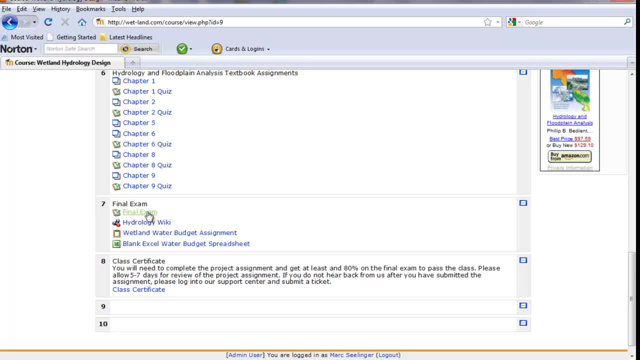 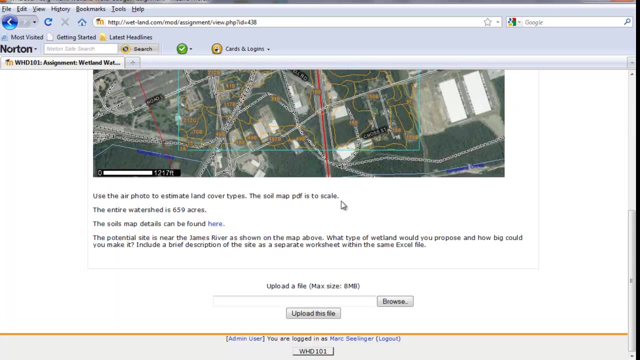 have a final exam, which is kind of a rehash of some of the quiz questions and some new ones. we have homework and this is the water budget assignment and what we basically have done is set up a sample project and you can see there's a site, kind of a location, here's potential mitigation site. where can 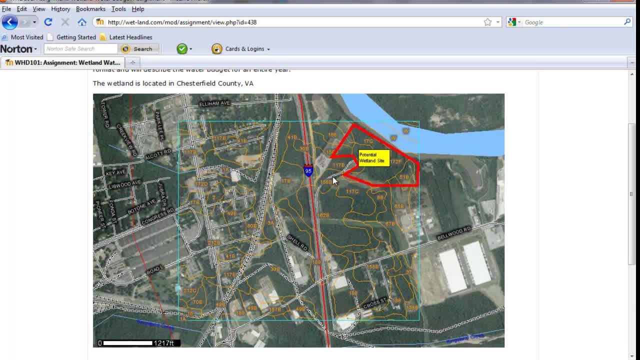 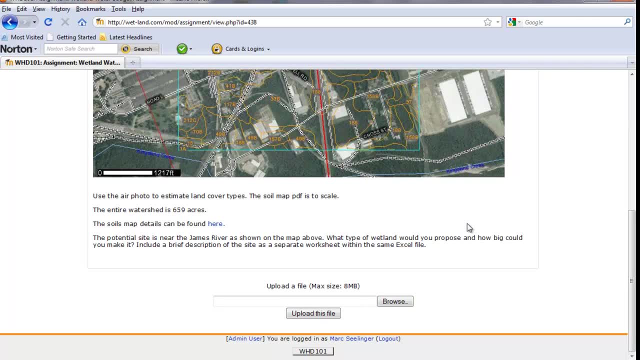 we find some more information about it and essentially, what we want you to do is to design a wetland based upon that, and what you're going to end up doing is uploading a spreadsheet which you can just upload it right into the site, and it's a. the spreadsheet is provided. basically what you're. 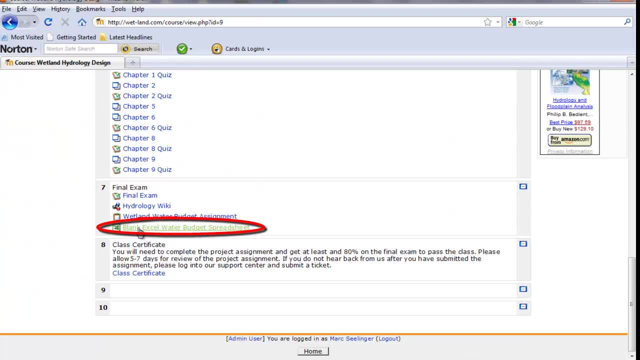 going to have to do is fill it out. so, and that's the spreadsheet for your, for your water budget, once you submit that, we take a look at it, and this is done manually, so this is not an instantaneous thing. we're going to take a look at it. we'll provide comments if we've got any questions or concerns. 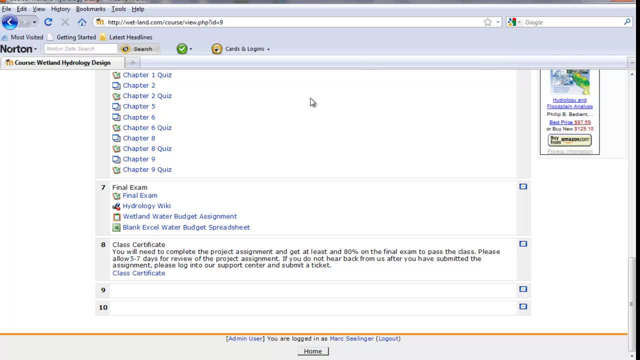 about what you've come up with. for example, if you've decided that the entire watershed is going to supply the site and we think, well, maybe that's a little bit over ambitious, give that's a kind of a heads up. by the way, maybe you need to take a look at where water is going, and so forth. so you 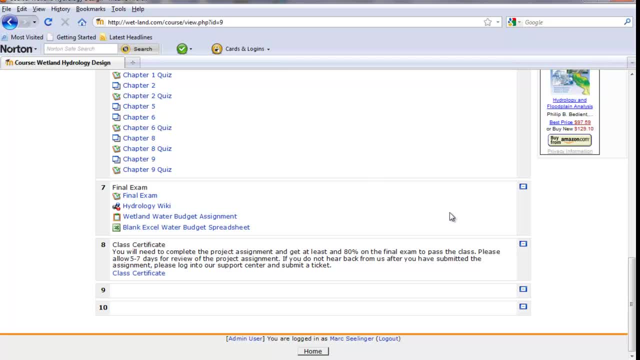 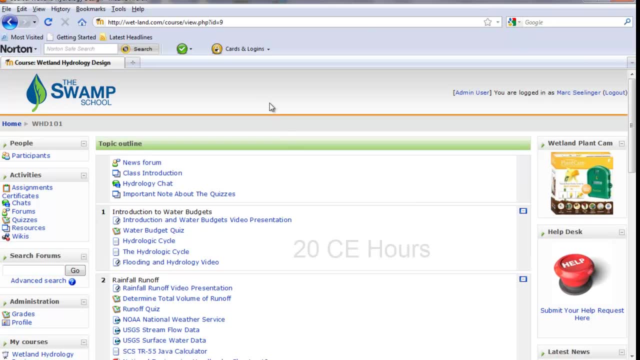 want to take a look at that and then submit your spreadsheet and you're good to go. once everything is completed, we issue you a class certificate. now this class has been approved by the Society of Wetland Scientists PWS program for 20 continuing ed hours. so if you're going for re-upping your PWS or you're going for PWS, this has been approved.